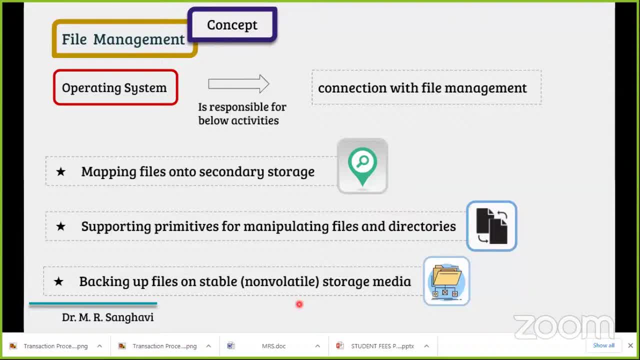 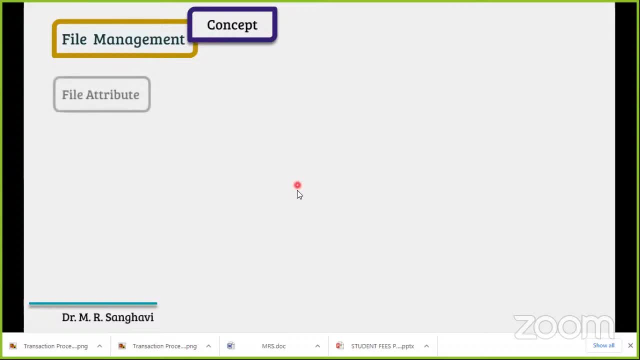 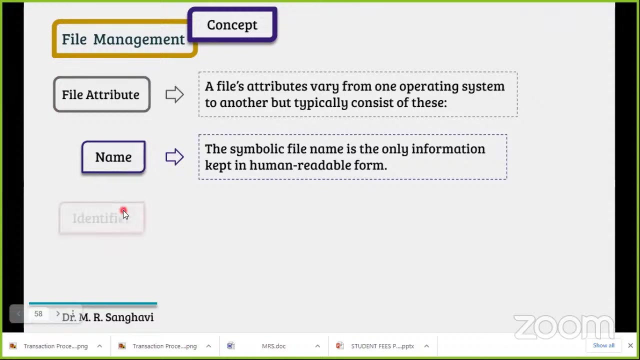 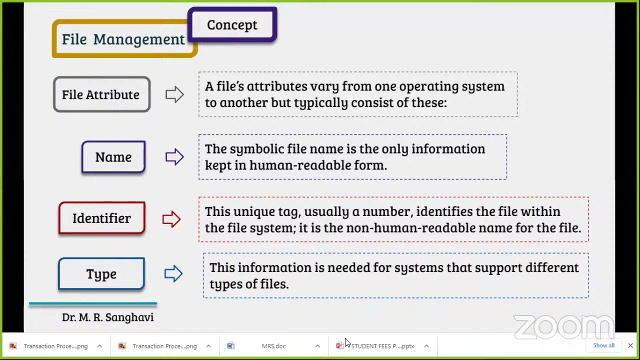 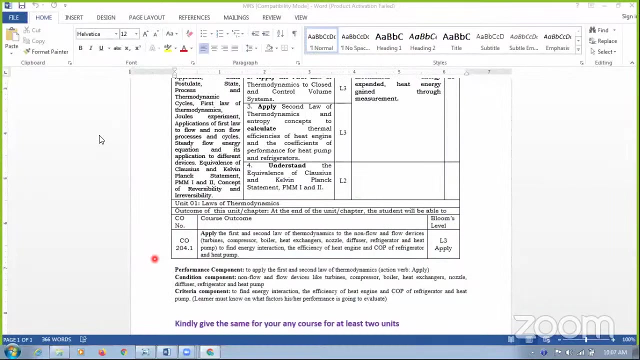 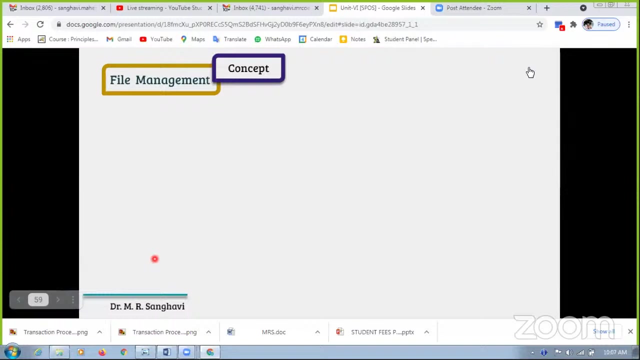 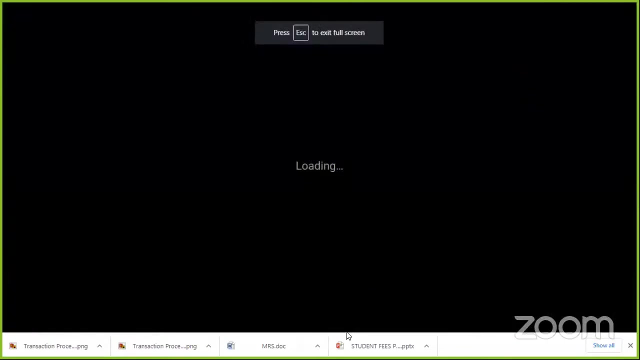 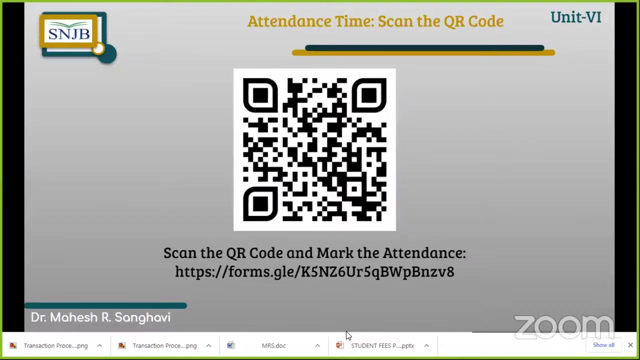 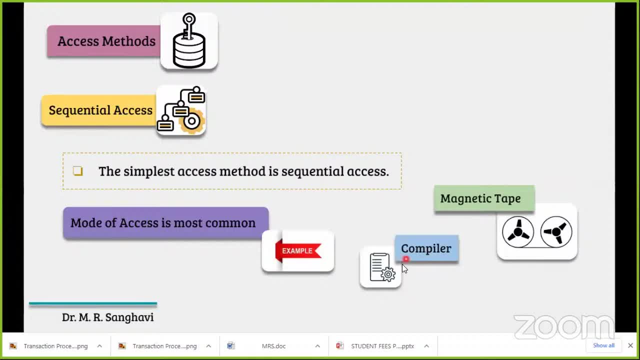 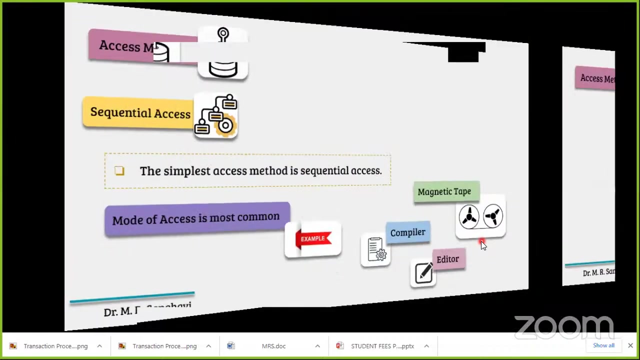 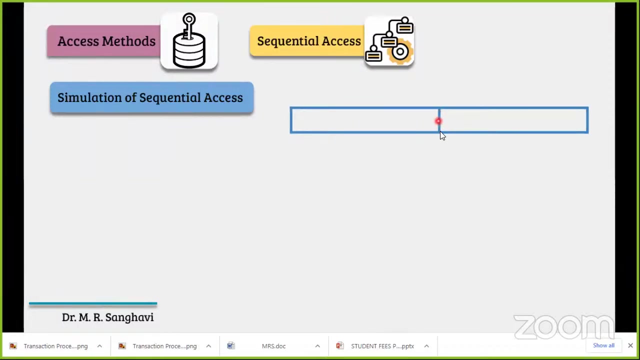 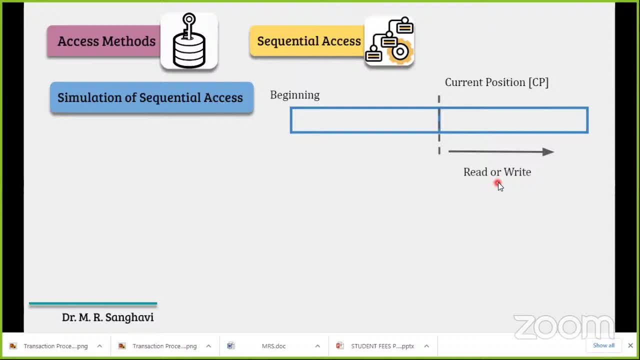 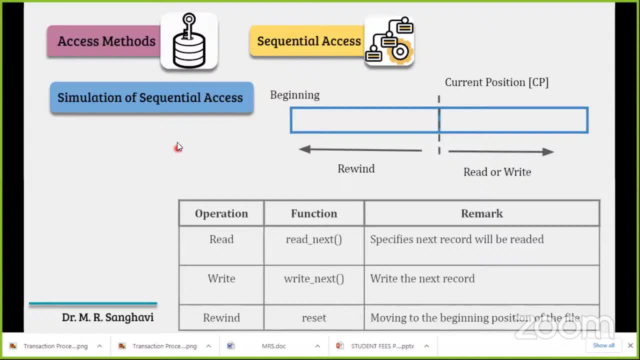 because this is not direct access. it is what sequential access that you need to understand. so what are the operations which are possible? read is possible with what read next, so you can either read next, read next. there is no read back option, there is only rewind means you can simply move. 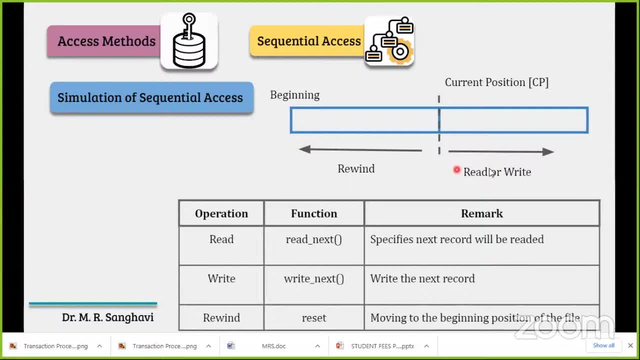 ahead. you cannot read the data. you cannot write the data. read and write is only possible with what read next and write next means you can go ahead. and what can you do with the records you can read? or what can you do with the coming records you can write? you can use this operation. 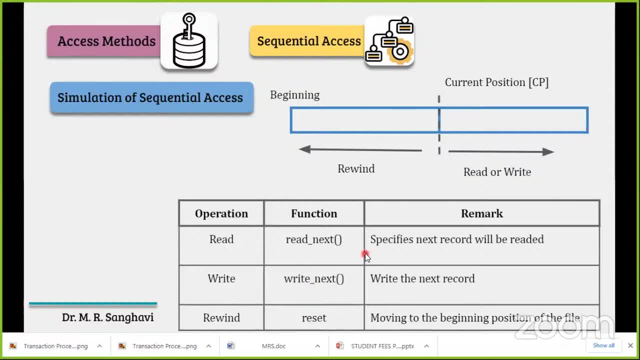 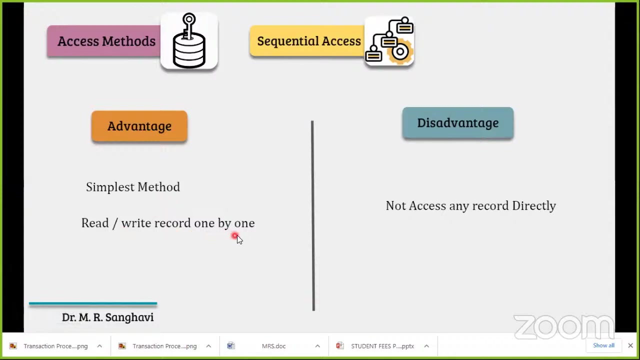 rewind here to go back side. rewind is only to position your pointer, file pointer to back side. okay, it will not read the data, it will not write the data. for read and write, there is only one operation, that is, read next or write next. and advantage: as i have already told you that it is simplest method: read, write, record one by one. 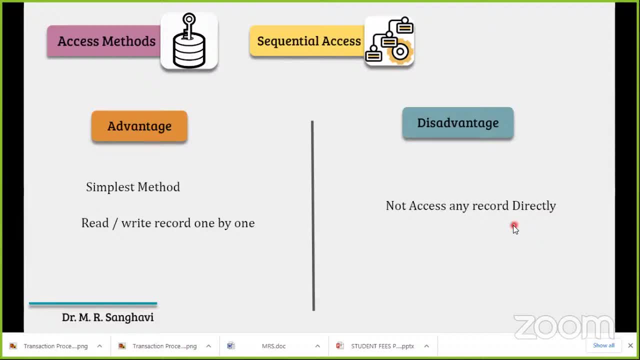 not access any direct, any record directly, so it goes sequentially. so it is one of the slowest. that is the biggest drawback of this sequential access method. many times in the university they're asking you what are the various file access methods or various types of files? you need to explain here sequential access as well as what direct access. so let's. 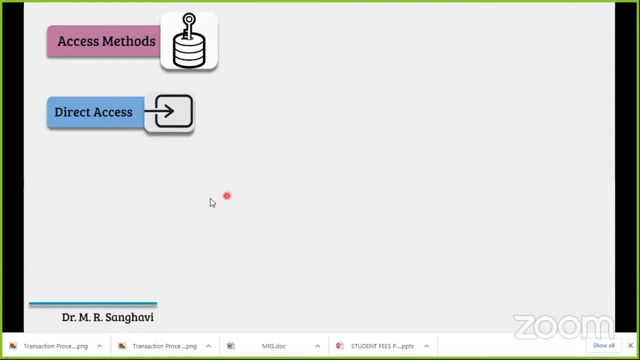 look at direct access. direct access, as the name suggests, you can implement this by using- you know, by using any, any side of any, any use of what array where you can directly jump to a particular record. direct access is also called as relative access or random access. both the names are same: random. 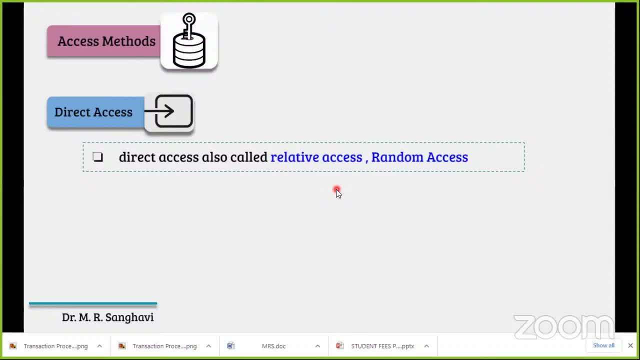 access or direct access. why the name random access? because, randomly, you can access any sort of record by using this direct access. hence the name are direct accesses. so let's look at direct access. so let's look at direct accesses. so let's look at direct accesses. so let's look at direct accesses. 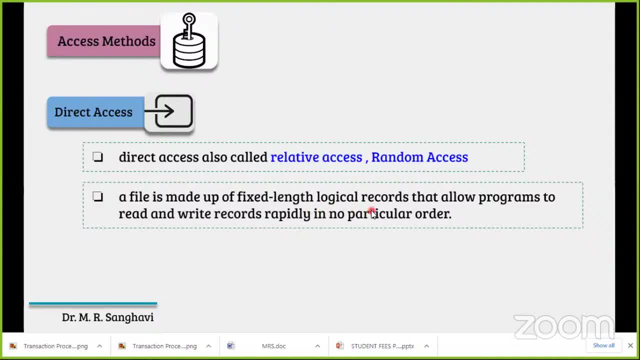 a file is made up of, you know, fixed length logical records that allow programs to read or write records rapidly in a particular, in no particular order. there is no specific order because it is not sequential. that's the reason it is known as what direct access, the direct access method is. 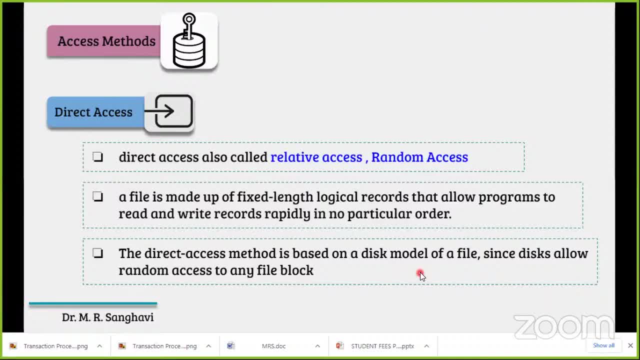 also based on disk model of file system, since this disks allow random access to any file block. nowadays, in hard disk, whatever data we are accessing, it is always a random access, it is always a direct access. so, whatever if you are implementing nowadays, whatever data we are reading, 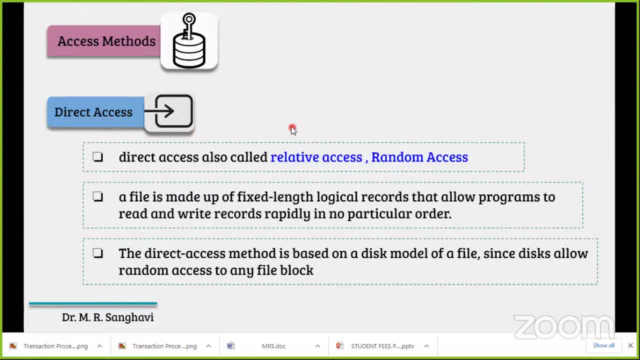 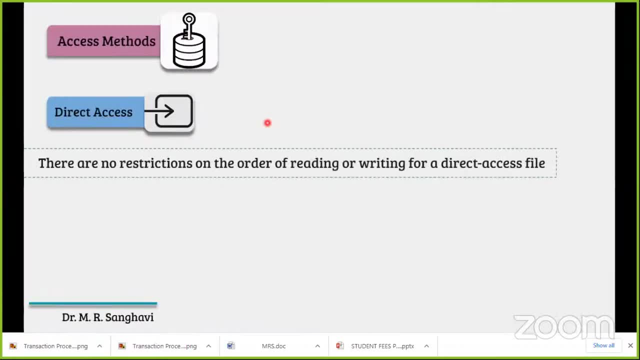 from hard disk. it is based on what direct access, so it is currently in use in our operating system so that you need to understand now, looking towards what there are. there are no restrictions in order. you can either read in any direction, write in any direction, or you can read in any direction. 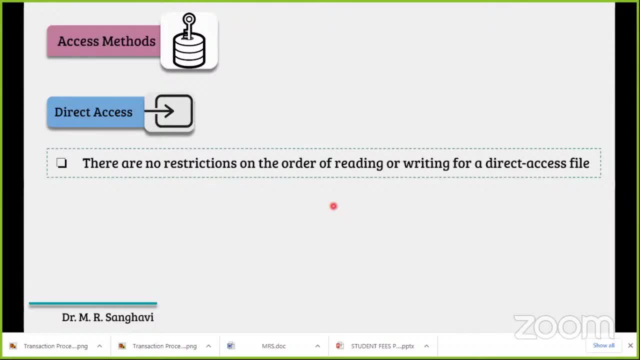 the way, in case of sequential access, only read next and write next were allowed. okay, but in case of direct access file, you can. there is no restriction. you can read anywhere, you can write anywhere randomly, you can jump to any of the record and you can perform read or write operation. for example, you can see. think about the magnetic disk means your hard disk. 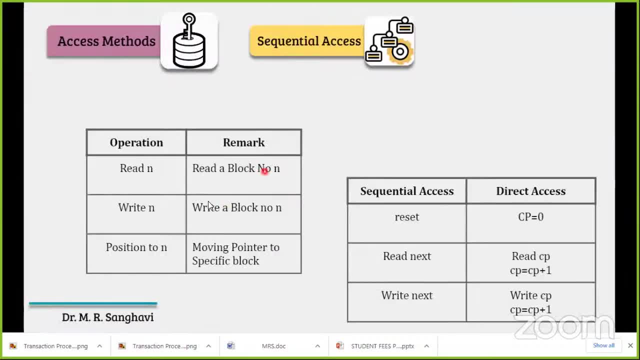 is the best example of direct access. these are the operations which are possible before direct access. uh, it is by mystic. the name is what copied. okay, you can see that access methods. here this is direct access and here it is what the sequential axis. now you can see that read n means what read. 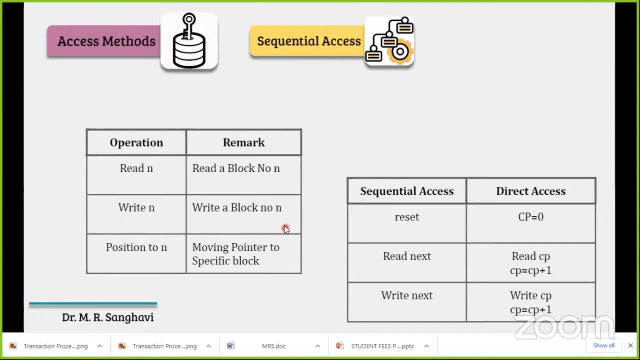 a block number n. write n means write a block number n. for example, if you say that, read 10, it will read the data which is available on block number 10.. write n means it will write data on that particular block number 10.. position to n means what you can jump towards, what that particular. 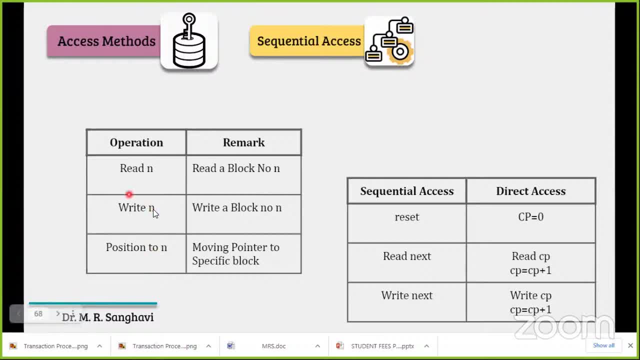 block. so that is the use of position. so you have, we have seen these operations like read next, write next and then what? rewind? rewind and position is one and the same thing. in case of sequential access, reset is what one of the operation where your file pointer will make. 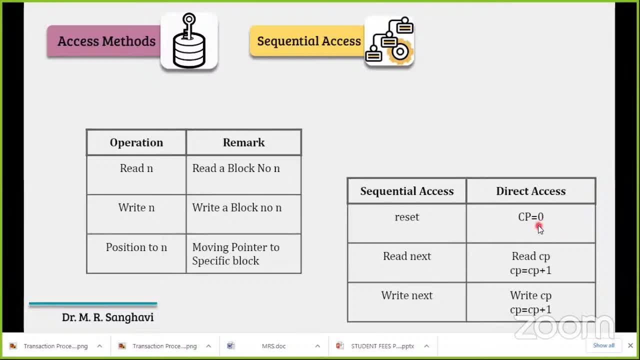 to what it is. it is positioned at start and that's the reason it is initialized to zero. here it is reset. here in direct access you can make it as zero. read next here it is ultimately read the value of cp and then you can just increment the pointer by one right. next is again: 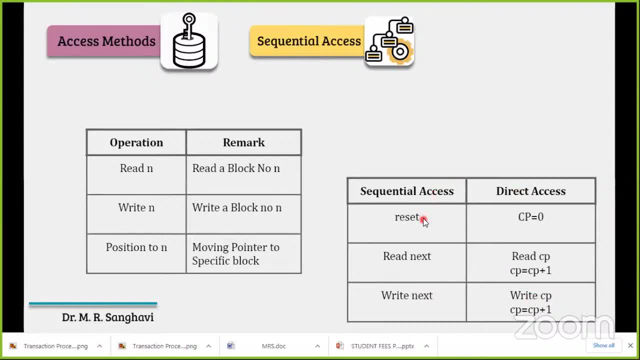 same like this. so in direct access sequential access can also be possible. you can even use direct access as a sequential access, but reverse is not possible. so we can say that direct access is more advantageous than the sequential access, and that's the reason it is heavily used in this particular industry, even nowadays. 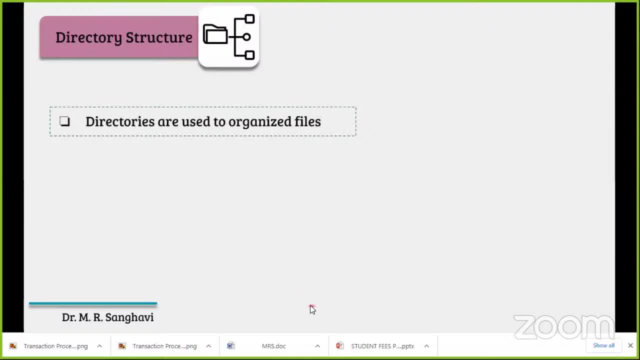 next point is directory structure. if somebody has any doubt, you can please raise your doubt. have you understood everything or am i going fast? are you able to understand? yes, sir, yes sir, okay, no doubt, no, sir, okay, fine, thank you. yeah, now directory structure. directories are used to organize files. okay, we can organize. 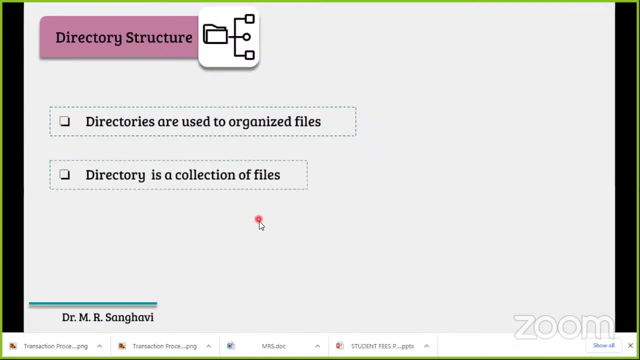 our files by using directory structure. it is collection of what- various files. we all are aware about what directory structures you know. we all are using windows operating system or linux operating system. we are creating directories and in inside directories we are actually what? storing files, various files, and that's the reason. directory is simply a collection of files. 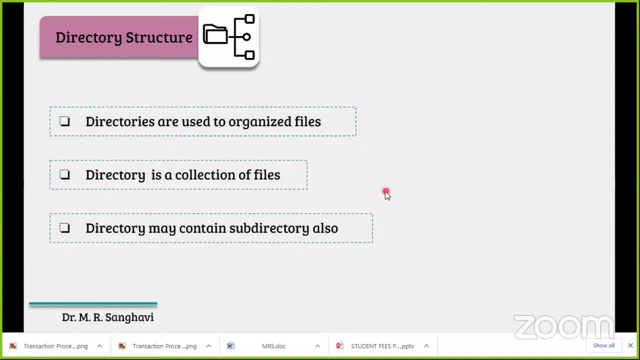 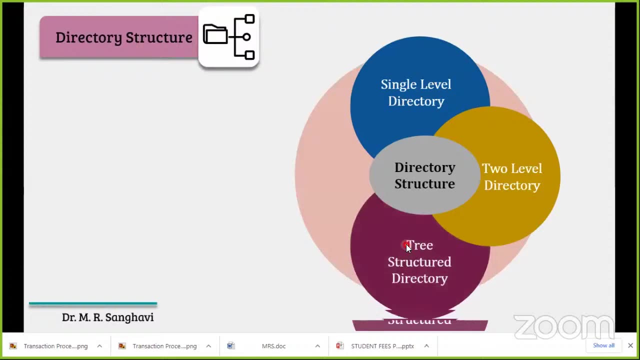 directly may contain sub directories. also we can create directories. under what directories? that is again what we have seen. there are various ways of what directly structures. okay, so, very first, one is what single level, then two level, then three structured directly, that is three level and there can be what a cyclic graph. 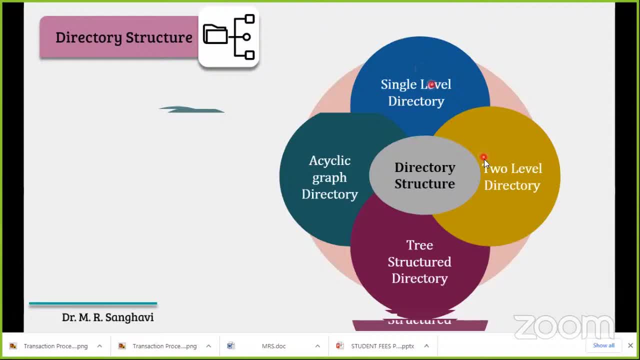 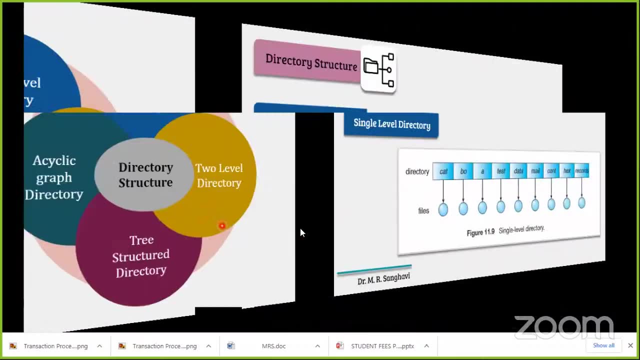 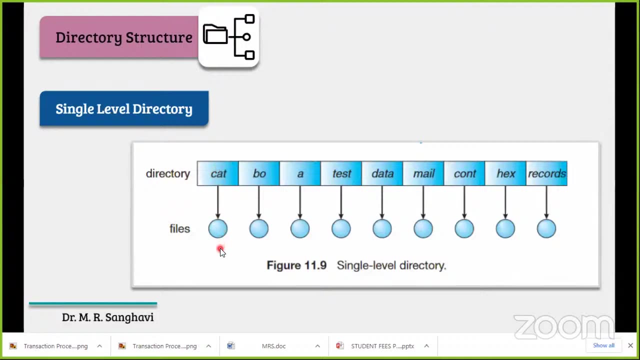 directory. so, dear friends, these are the four types, that is, single, double, third, three level and a cyclic graph directory structure. so let's look at one by one. single level means what we can able to create a directory and inside that we can able to store a file. so we cannot create directly. 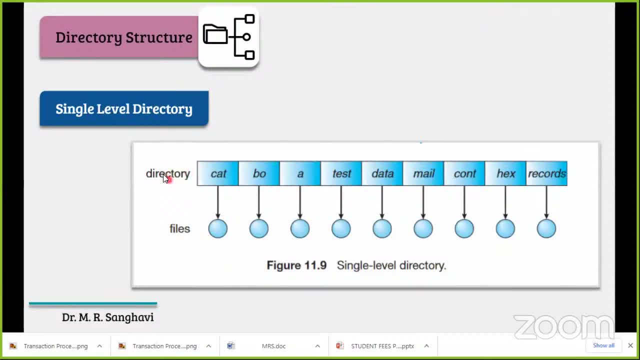 under directory, in this single level directory. okay, that is the issue. so directly will be only one. under that we can store the multiple files, that's not a problem. we can store multiple file, that's not a problem, okay, but we cannot create directly under what sub directories. 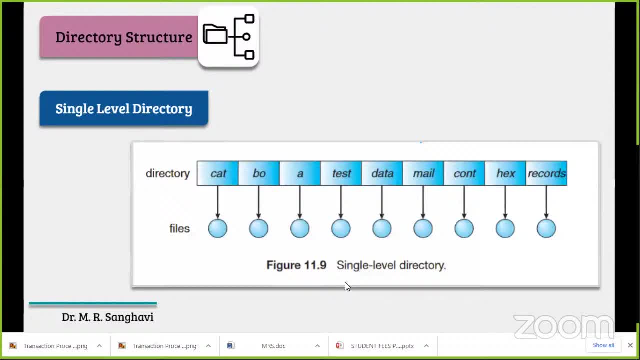 i hope my voice is audible to all. am i audible? yes, sir, yes, sir. okay, so several directory means what we cannot create directly under the directory. there will be a single directory under which we can store multiple files. so the simplest level of directory structure, because only top root means every- uh, you know, every- directory will be at same. 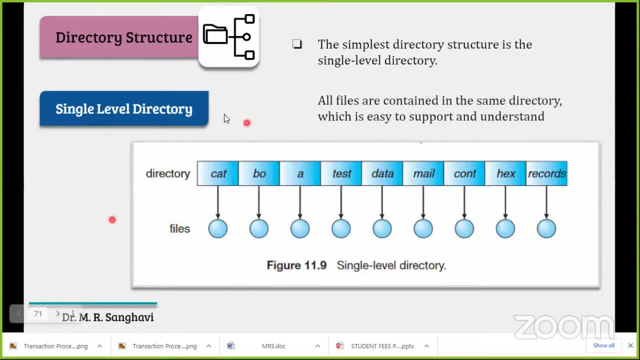 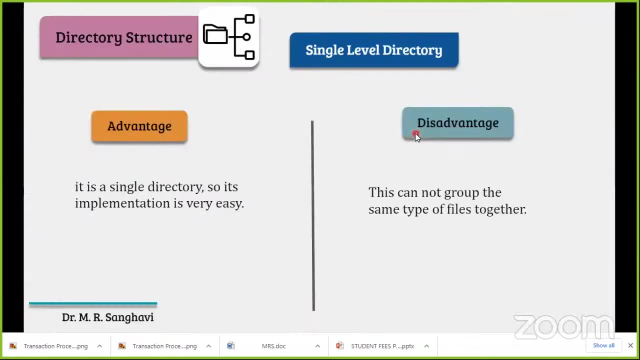 level, then we can see this particular part here, that folder, and there will be what, directly what? there will be files, so all files contained in same directory, which is easy to support and understand. now, the advantage: it is a single directory, so its implementation will be very, very easy. 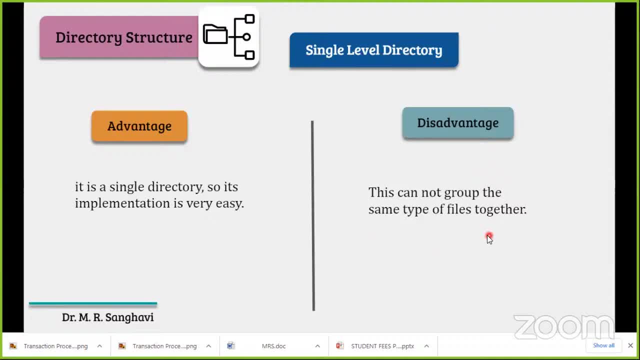 disadvantage. this cannot group the same type of files together. so as we all are aware that directory under directory will give us what various ways. for example, i'm talking about engineering. suppose engineering is one of the directory, and if we store data of all the students, okay, maybe computers. 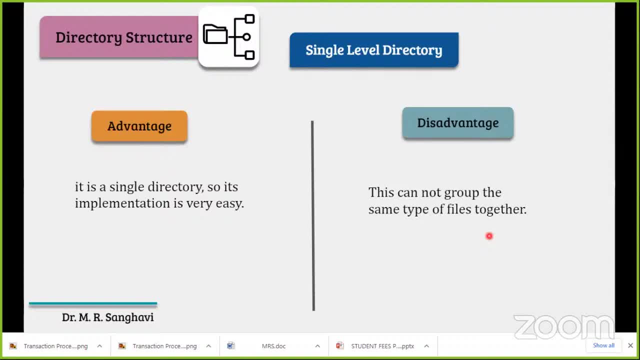 civil, mechanical electronics, all kinds of data will be stored. then searching will be difficult. so what we do is we can use a directory under directory, so under engineering we can create computer engineering, then civil engineering, this kind of directories and under which we can store data of computer engineers, civil engineers likewise, so directly under directory is important and that's. 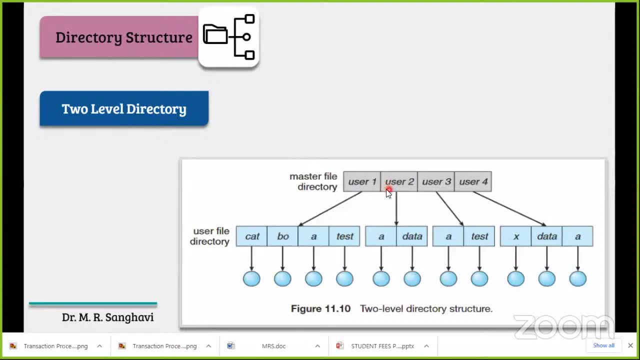 the reason we can see here two level directory. two level means what we can create: main directory and under that there will be one sub direct. so what will happen? you know. here we can. we can use one of the directory level directory as engineering okay, under which we can have subdirectories like computer engineering. 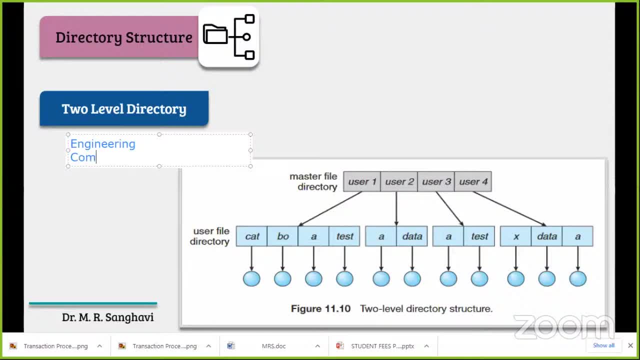 or it or maybe civil. likewise, we can create subdirectories, so these are what subdirectories under this main directory. okay, so one level can be possible, so we can create one sub directory under one main directory. but we cannot even go with what sub sub means at third level. it is not possible because its name indicates. 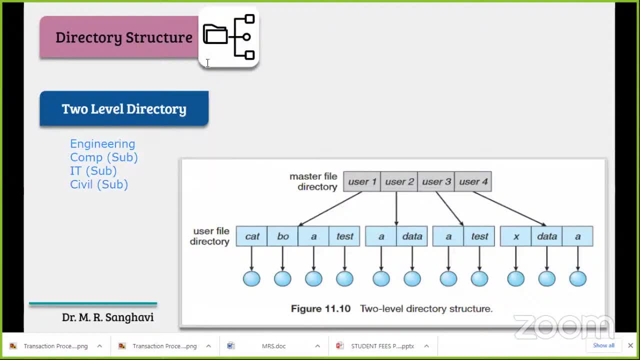 that it is ultimately two level directory. but again, if we want to separate out from computer, if we have to separate out like software and hardware and networking, in that case the third level is not possible because it's not possible to create a sub directory under one main directory. 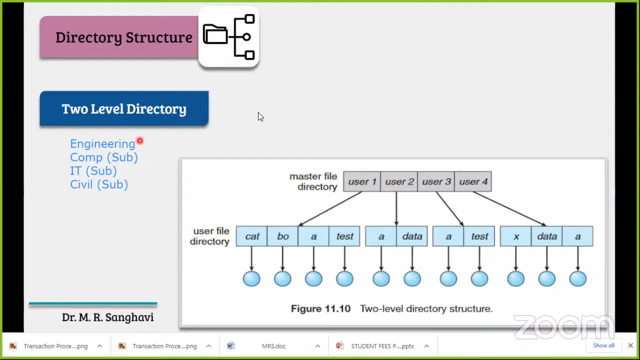 name indicates that it is two level directory structure. so two levels at max. it is what it is possible. okay, the way we are observing here, okay, so that is possible. but the beauty of this is what suppose the students which are at computer engineering cannot see the data at it cannot see. 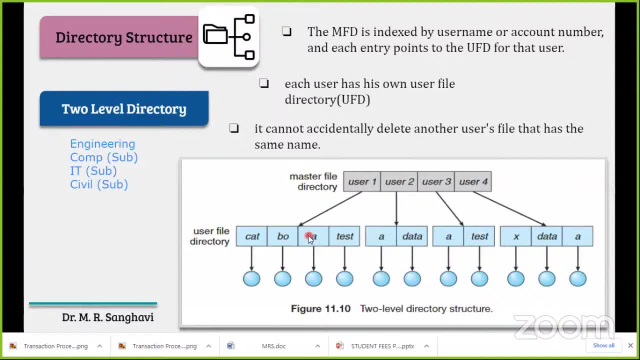 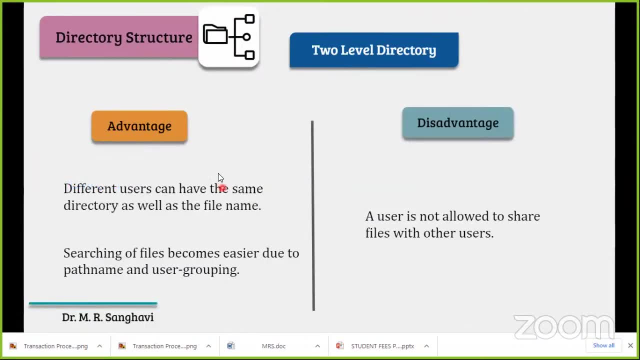 the data at civil. that indicates that you can somewhere use some kind of protection. that's the beauty. now advantage: different users can have the same directory as well as what file name. searching of file becomes very easy due to path name and user grouping. so if you you want to search data of all computer, 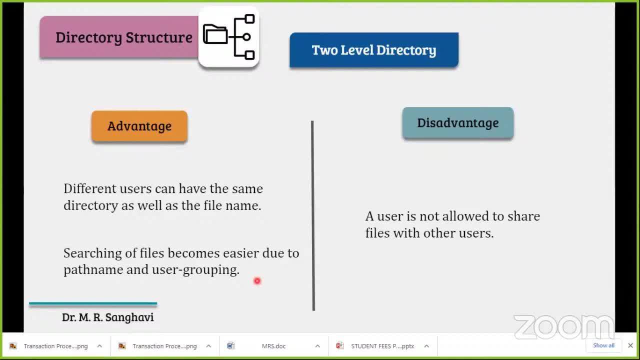 engineers, simply enter into engineering, then computer engineering, and you will get entire data, whereas, again, users are not allowed to share files with what other users, so you cannot. this is one of the drawback, though it is one of the protection thing, but it is one of the drawback. nowadays we are sharing data from one directory on another one. 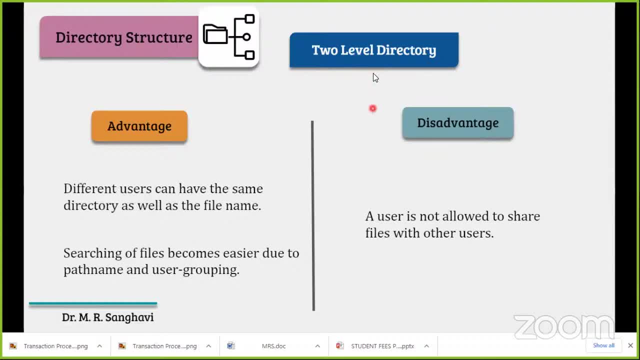 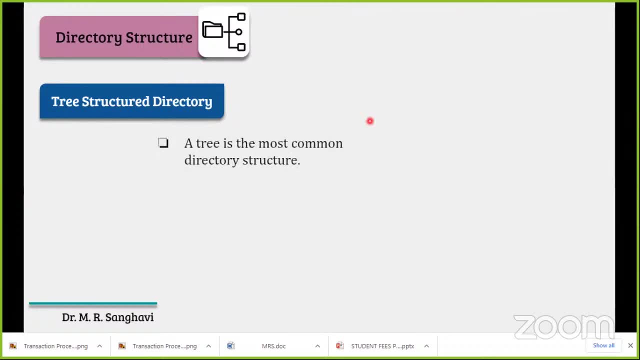 to another directory. that is not possible in case of your two level directories. now the next part is pre-structured directory. pre-structured directory means what? there will be multiple nodes inside. okay, so the tree is most common directory structure. we all are aware about this, right you? you have seen this pre-structure in case of even windows explorer. windows explorer. 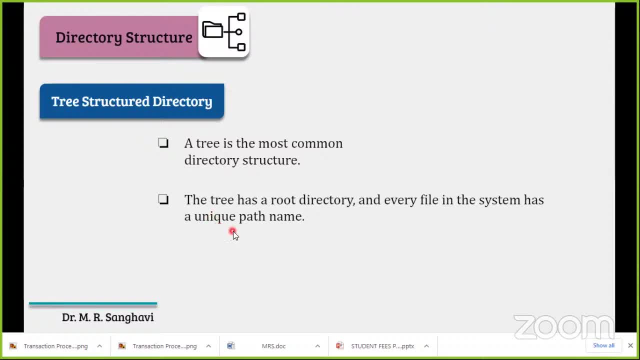 is ultimately what one of the tree structure, that which is given, so data, you, you may get that plus sign and the way towards what we are expanding that entire data. so the tree has one root directory, so it may start with c colon, d colon or any of the type okay, and every file is accessed. 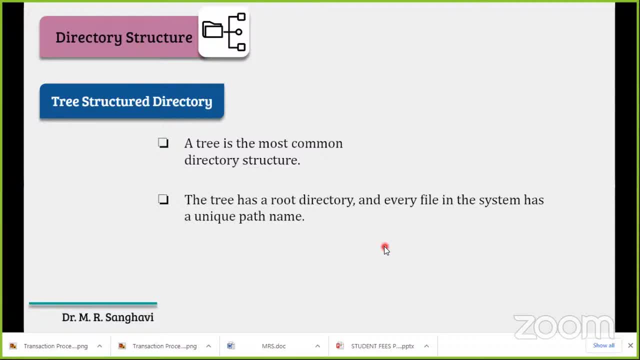 with what unique path name means we are using drive, then name of directory, then name of what file. this way we can able to access any of the file by using its partner, unique partner. every directory or sub directory contains either set of files or sub directories. so every directory can means there is no restriction here. 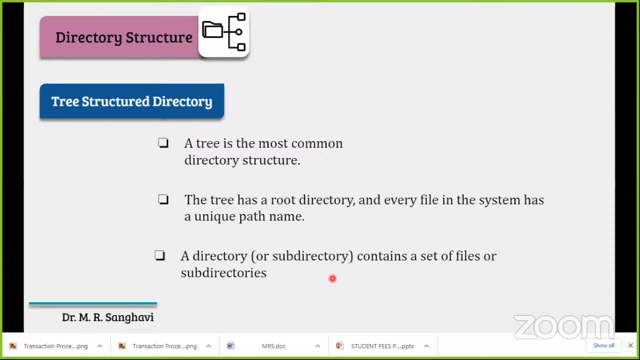 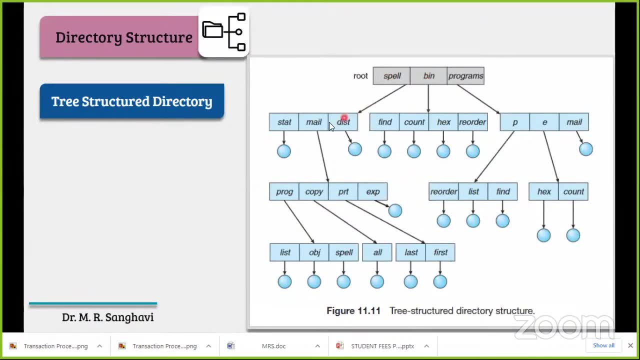 so ultimately directly may contain files or sub directories, and this is what the structure that you can see here. there is no restriction. you can take any directory under any number of directories. so this level- there is no restriction of what level- and this is the most prominent structure accepted heavily into what market and steel windows. 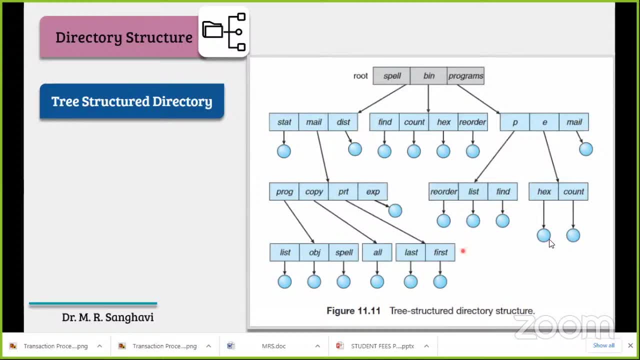 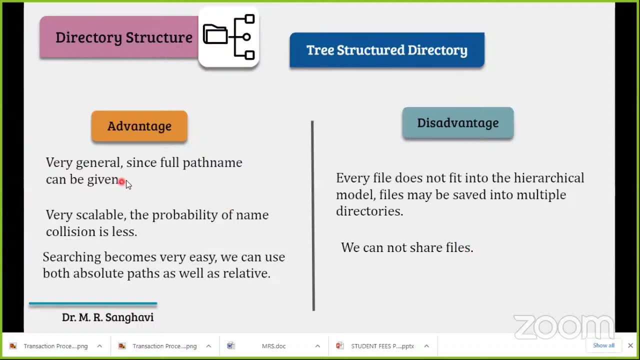 microsoft is also using it heavily, so that you need to understand now the pre-structure also has its own advantage and disadvantages. it is very, very general that we have seen, in even windows and other operating system, very scalable. the probability of name collision is very, very less because, though, you have to give the same name of file, but you can mention, you can store. 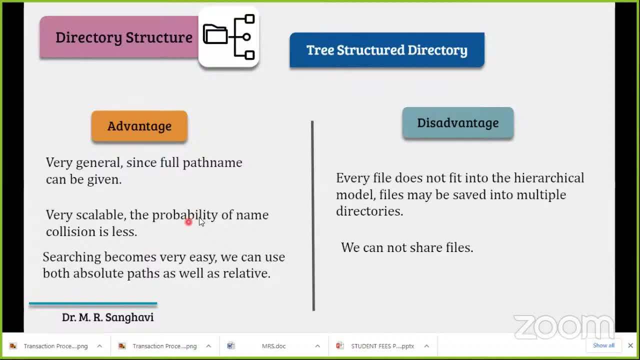 it into what different directory or different folder. then you can even use the same name, so the collision of naming will be very less. searching becomes very easy because there will be multiple path will be. there will be absolute path or relative path, so searching will be very, very easy. 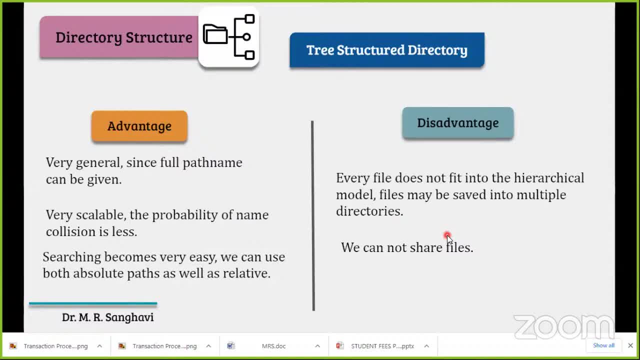 the disadvantage You can see here. every file does not fit into hierarchical model. Files may be saved into what multiple directories Same file can be saved into what multiple directories? So problem will come and we cannot share the files. That is again the biggest drawback. 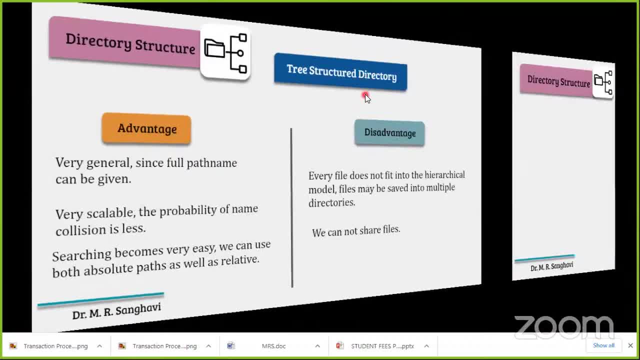 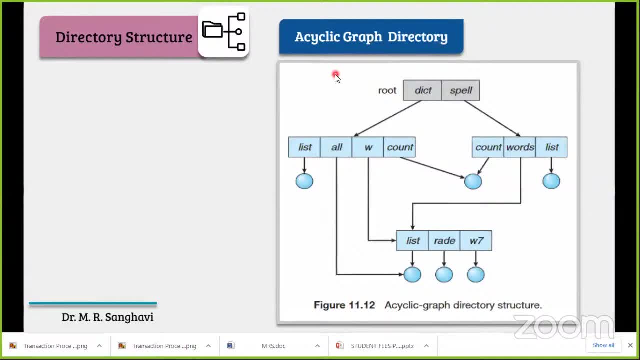 of what sharing in case of tree structure, And that's the reason nowadays a cyclic graph directory is used. A cyclic graph means what It is: a graph which won't have any sort of cycle. A graph which won't have any sort of cycle. 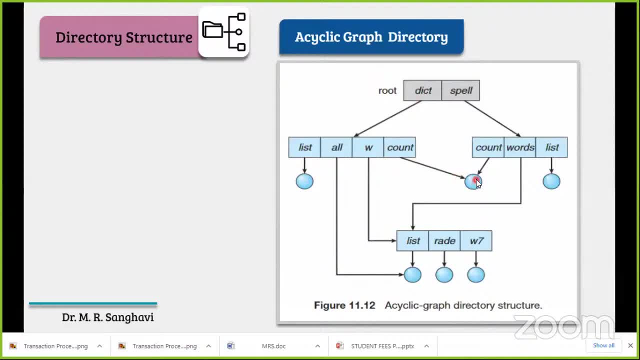 If you see here, this came here. this came here, but this one is not going here. this is also coming here. This is also known as what a cyclic graph. But what is the beauty of this? This one is a common file. 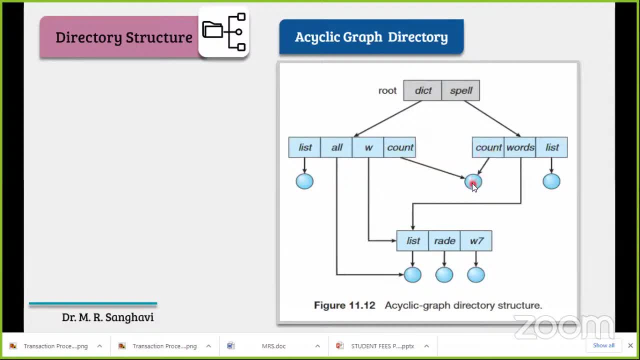 which is common for both these directories. That means we have shared from here. So sharing is possible. in case of what this kind of directory structure? So, dear friends, we have seen four types of directory structure. One single, where only one directory creation is possible. 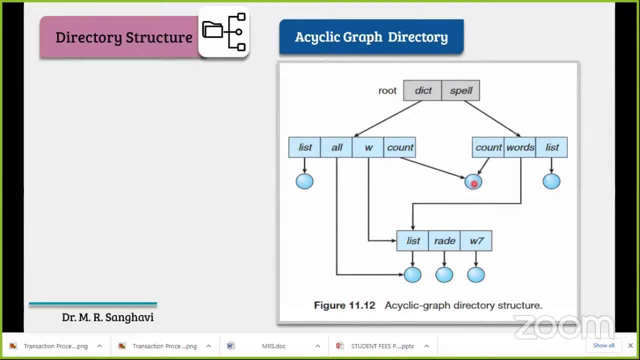 Two level where two kinds of directory creation is possible. Then we have seen tree structure: No level. you can go with any level, but only drawback were what sharing of file? And that drawback is removed in case of your a cyclic graph. 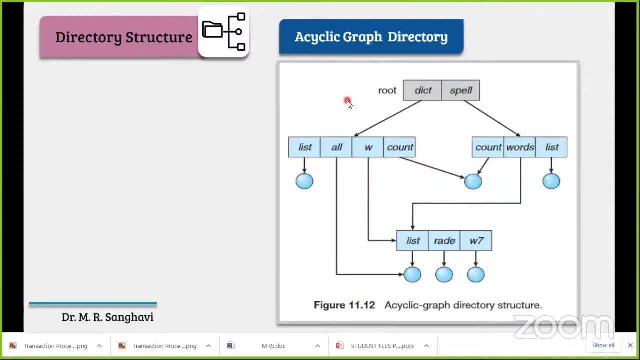 So a cyclic graph is actually your. it's like tree structure, but having cycle where you want to share what. So it has one of the option, like sharing of file. But always remember it is a cyclic means there will not be any sort of cycle here. 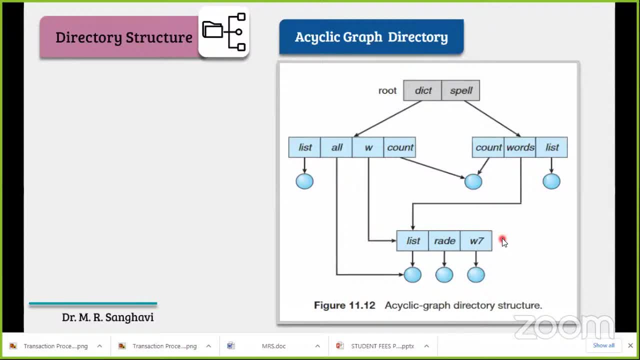 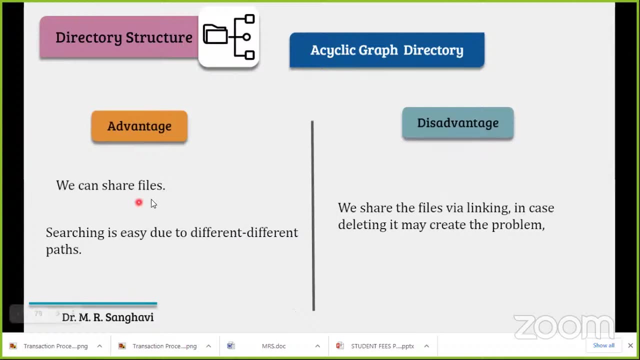 So that you need to understand- And that's the beauty of a cyclic graph- directly And these kinds of things that are used in the market till date, So you can see all the things that I have already told you. It's advantage we can share the files. 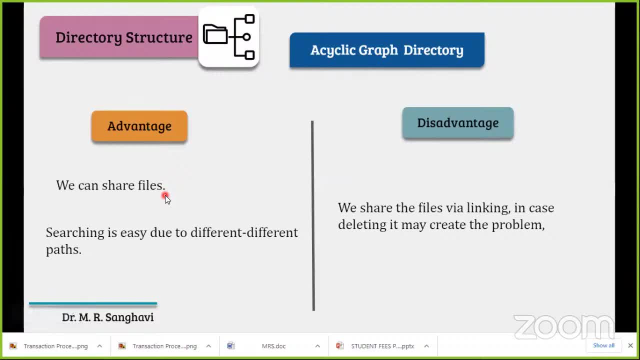 Yes, it is possible because we have seen that particular path. okay, Searching is again easy. We share the files via linking. In case of deleting it may create. what The problem? What is the problem of sharing? Suppose this file is deleted? 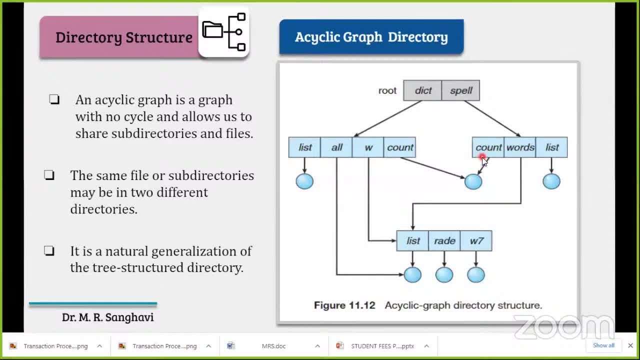 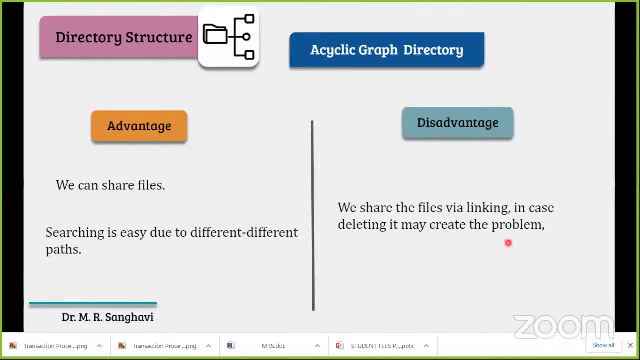 Suppose this count has deleted this file, So this will also go out from this particular count, So this will not be available. So sharing can be what Dangerous here? So every, you know, every method has its own advantages and disadvantages that we have seen. 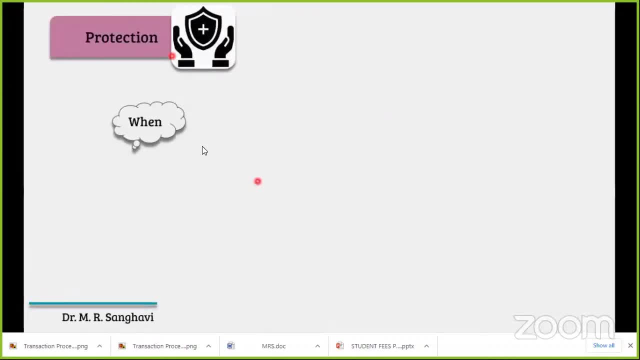 And that's we need to study always. Now the next part is protection. Protection means what We need to protect our files So that people won't be able to write on it. People, if we want that, we don't want to give any sort of access. 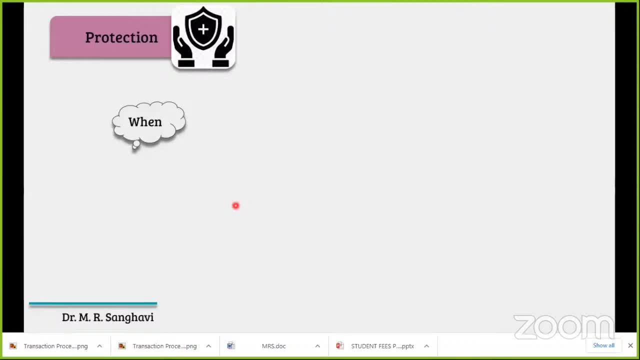 that can be even taken care. into what protection? Ultimately, the content of file should be what Untouched, And file should not be removed by anyone. So protection means what it is that information is stored in computer system. We want to keep it safe from physical damage. 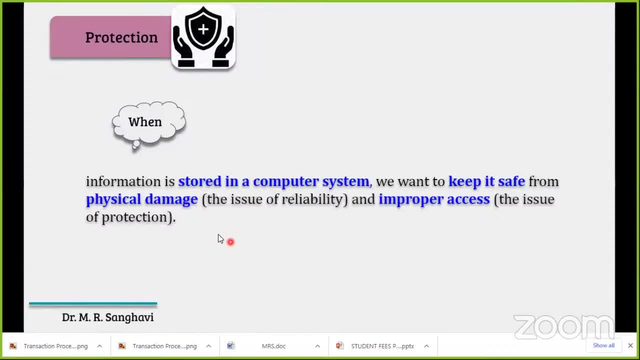 The issue of liability and improper access, the issue of protection. At that time floppy disk had been used, So the floppy disk had come out of the computer and in the next computer floppy disk used to get damaged. So physical damage it took was also there. 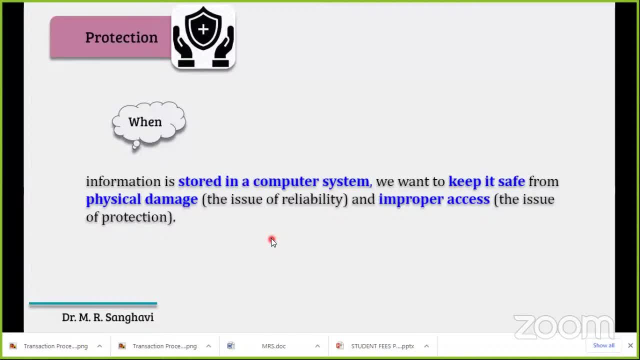 That was the biggest problem during those times. So now, in today's date, it's not a major issue. Still, the people who have a problem in Hard Disk that bad sectors have come look at their data. it does not work. 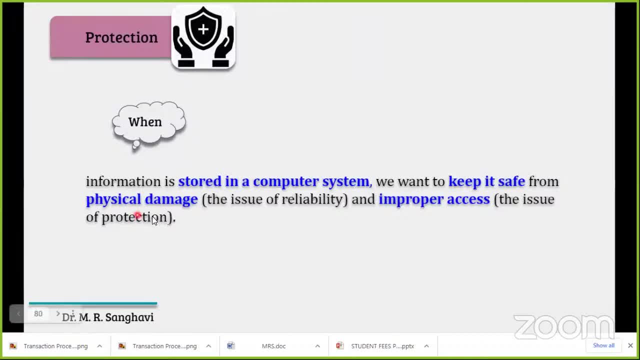 So that is ultimately what physical damage Like. you seen that. So operating system is actually taking care of this protection. You must have seen the CHKDS command. We check the disk and try to remove the bad sectors or patch up them. 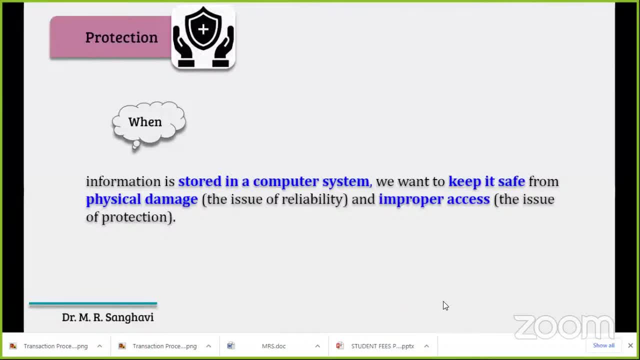 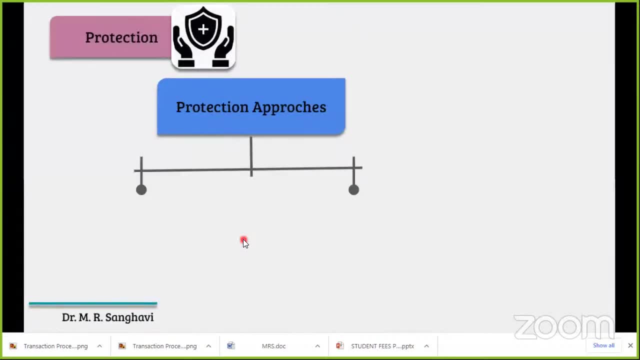 so that the information will never be stored there. So that is what the biggest concern when we are talking about the protection. So protection approaches are basically two: Prohibiting access and free access. that is no protection. Prohibiting access means what? 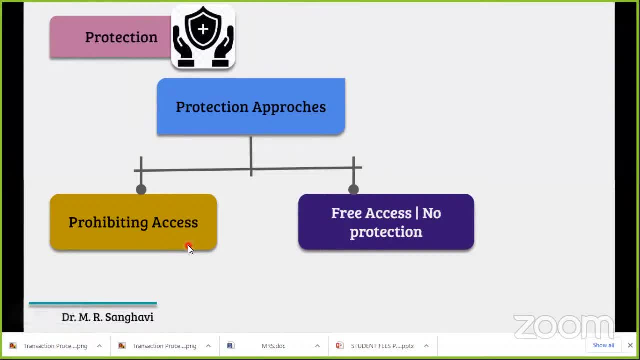 Either you will give the operation of read and no one will be able to write in it, or you will give write and not allow to execute. So these are the operations that can be possible, that is normally known as prohibiting And what is free access. 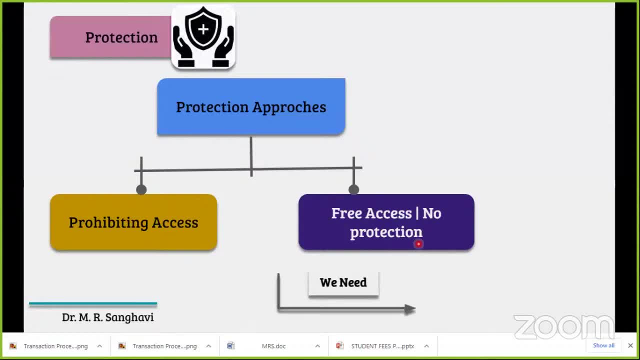 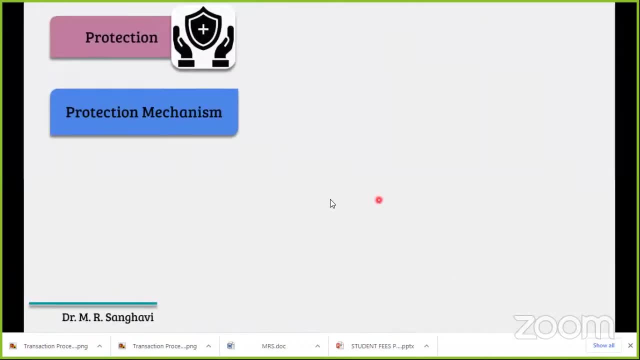 Whatever you want to do with the entire file, there is no protection. But how will it be done? So we need to focus on controlled access. So what is controlled access? So let's focus on protection mechanism. Protection mechanism is actually providing you what? 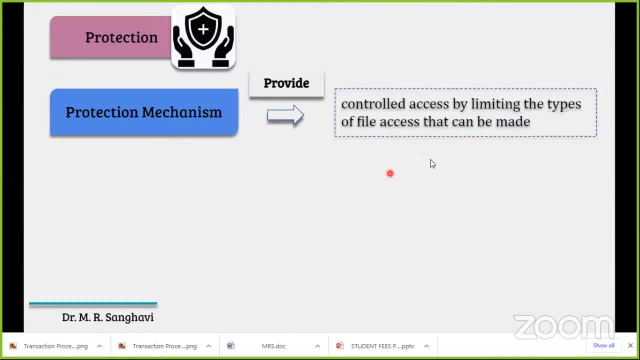 Controlled access by limiting the types of file access that can be made. Okay, So access is permitted or denied depending on what Several factors. If you think that there are students of the same group, Okay, You have seen many times that your seminar group is formed. 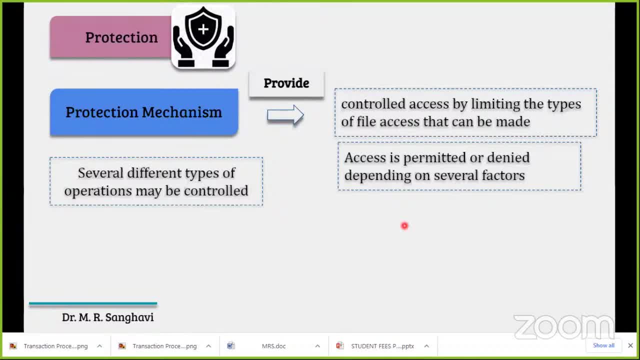 If the seminar group is formed, then there are 3-4 people and there will be your guides with you. So you must have given the operations of write to them. But the other members, like your seminar coordinator, you think that you have to share that file with them. 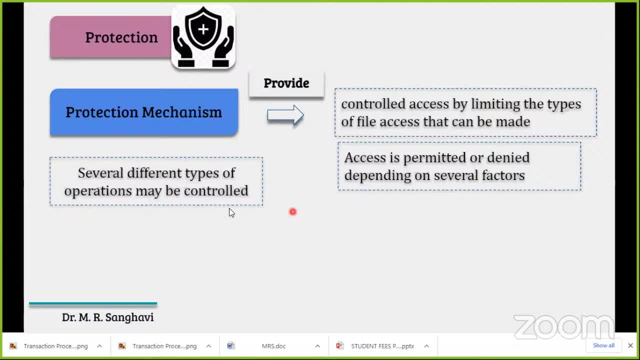 But they should not make any modification in it. So what do we do? We give them the rights of viewing by accessing read only. We don't give them the rights of edit. So we give them the rights of viewing. That is ultimately known as what? 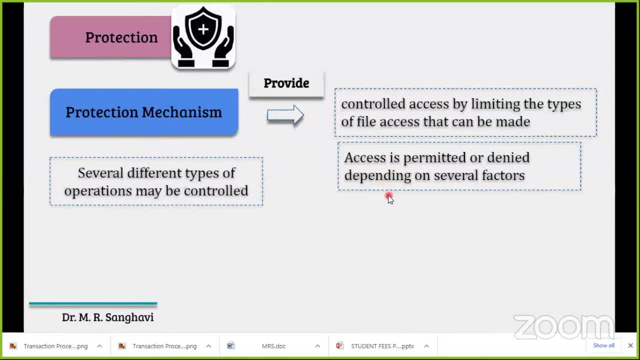 Access method. Okay. So what are these access rights? Read, write and execute. These are the 3 types of access rights that you need to understand. Several different types of operations that may be controlled will be what Read, Okay. 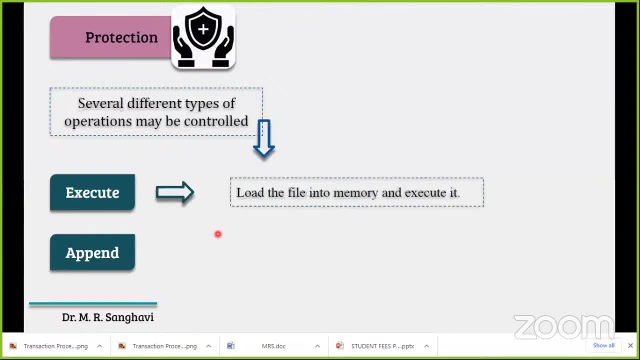 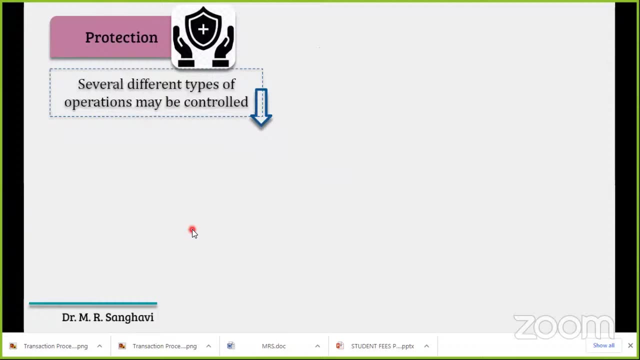 That is read from the file, Then execute And append. That is ultimately what Write: information into what File. So this I have already told you: Read, write and execute. Append is ultimately write, because we are always writing at the end of file. 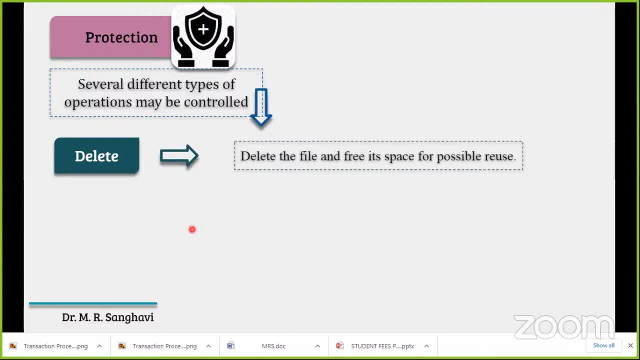 Even there are some certain different operations like delete. We can even not give access to delete so that people can't able to delete your files, So that is also possible. Provision is there. Okay, Then the list. that is ultimately what. The list, the name and attributes of what. 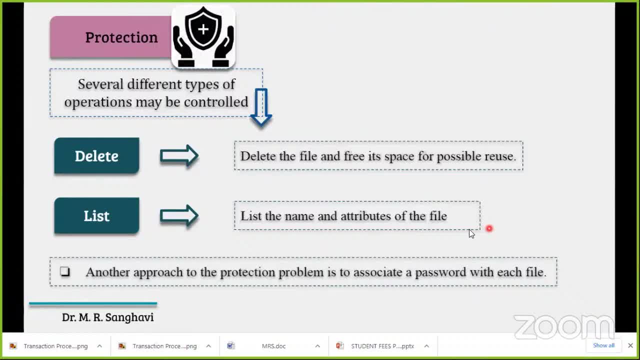 File. So these are the issues. Now you must be aware that you are actually what. What happens with your windows file? What do you do? Some people download a software of file protection that protects the folder. What you people will do to that folder. 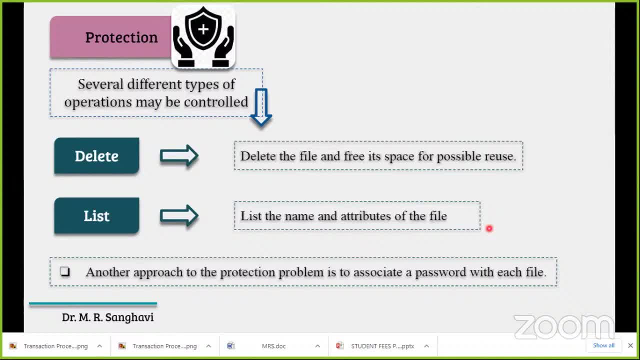 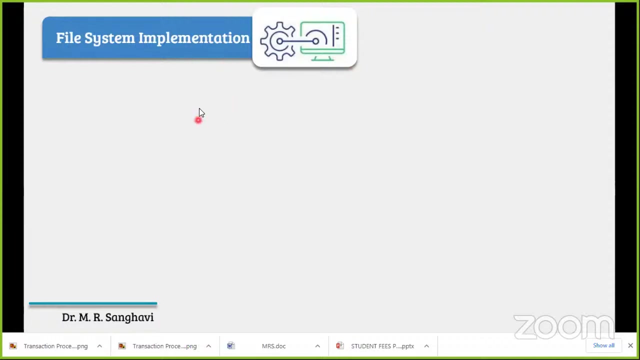 A password will be added Whenever someone opens it. Then go and open it, but you can always use third-party software for more protection, and operating system is supporting that. now, the last topic of today's session is file system implementation. we can, you know, we all are aware that file is collection of information and 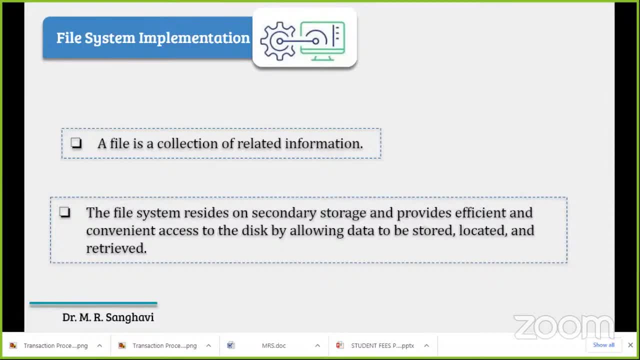 the file system resides on secondary storage and provides efficient and convenient access to disk, allowing data to be stored, located and retrieved. so we we must know, while implementation, what is file and what. what are the operations that we need to implement. dear friends, i'm happy to inform you that you all have implemented file system implementation and we will be. 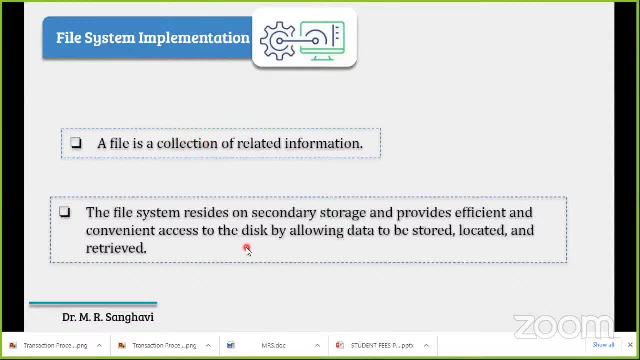 working on it in the next few days. so thank you so much for your attention and we will see you in the next session. bye, bye. file. in case of data structure, you have already the file. you have sorted the file. you have searched the information in a file. 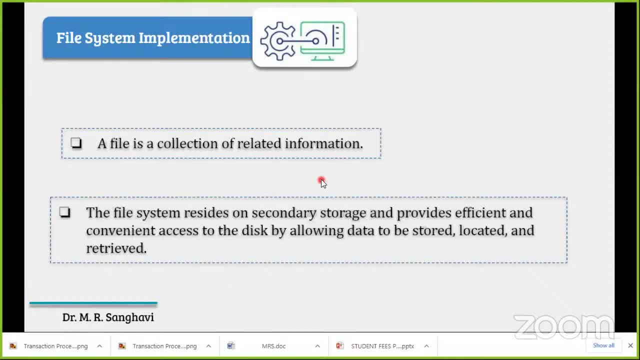 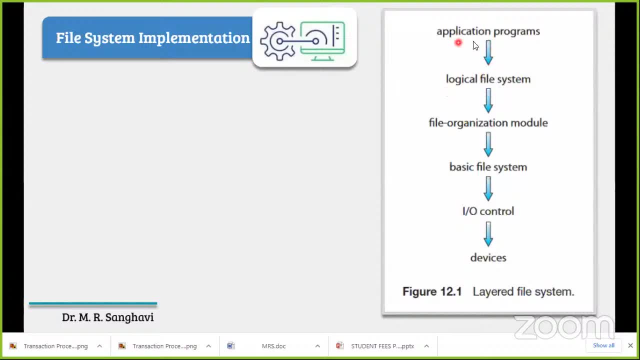 so that's the part that you have already implemented, while your dsf, that is data structure, practical. you need to understand here there is what application program which will access application program, manager, program upload, upload in c, c, plus, plus. well, is the layered system that you need to understand. so this is what, the basic file system where we can.